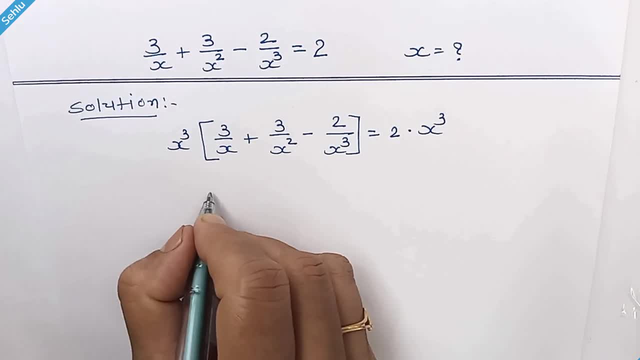 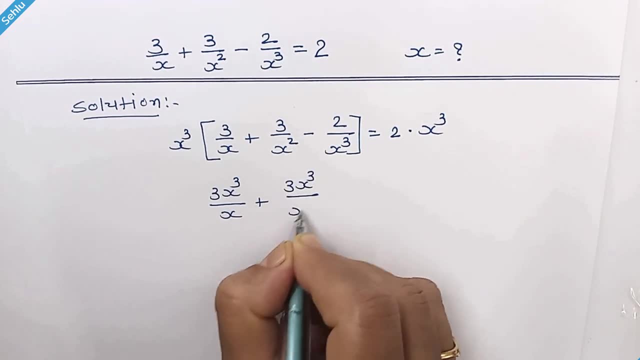 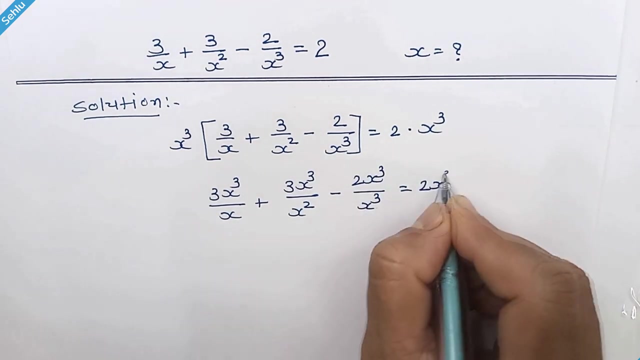 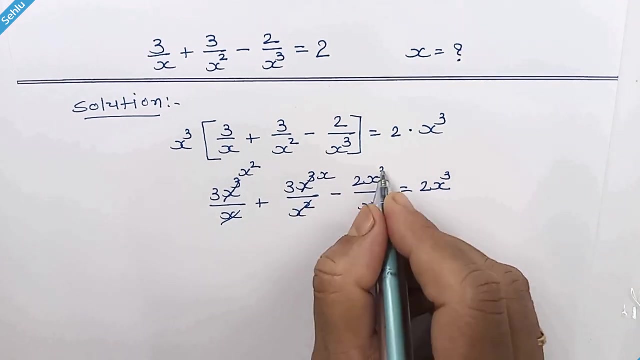 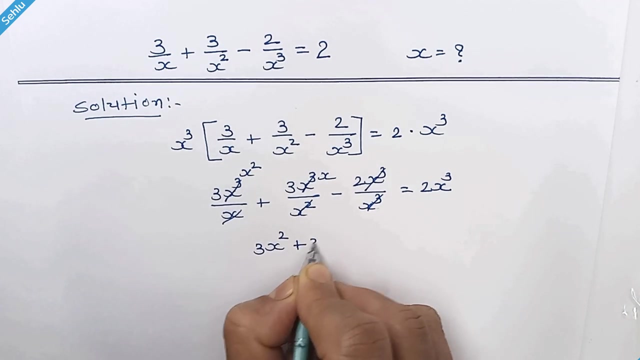 Plug in this x cube into this bracket. So here we have x square, here we have x, and these two will cancel each other. Now we have 3x square. plus 3x minus 2 is equal to 2x cube. Move these two here on right hand side. 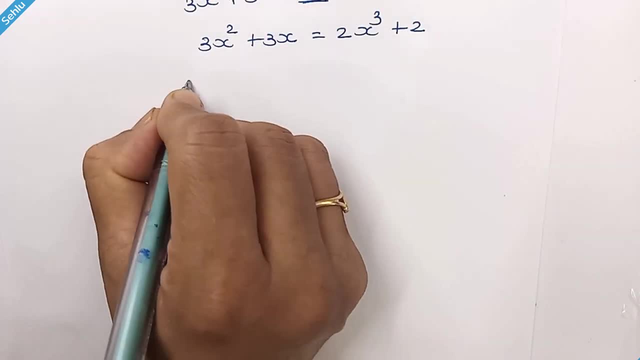 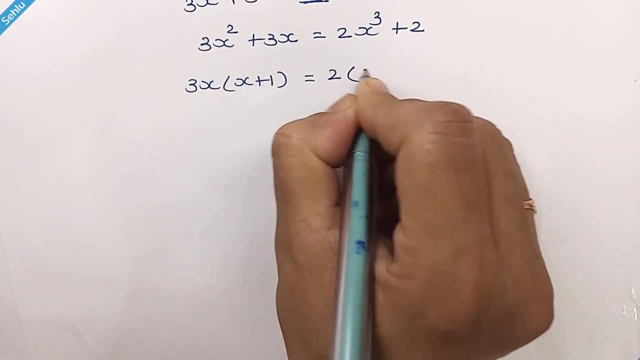 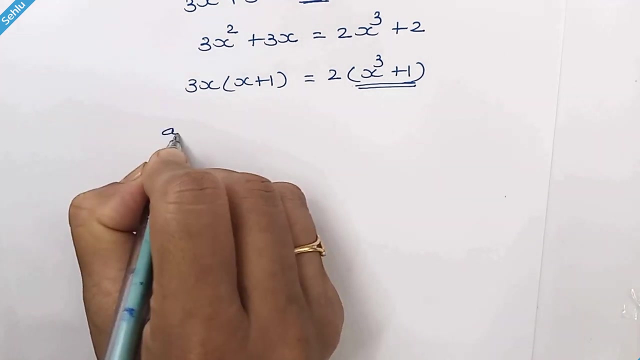 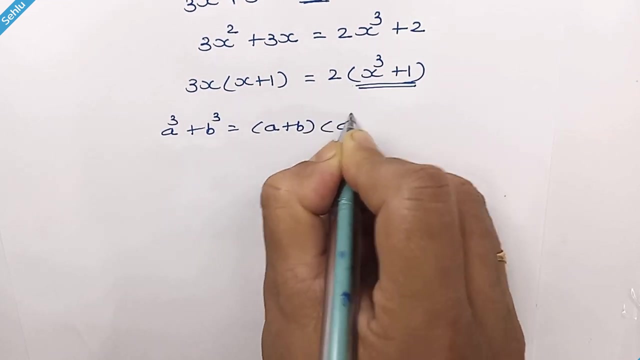 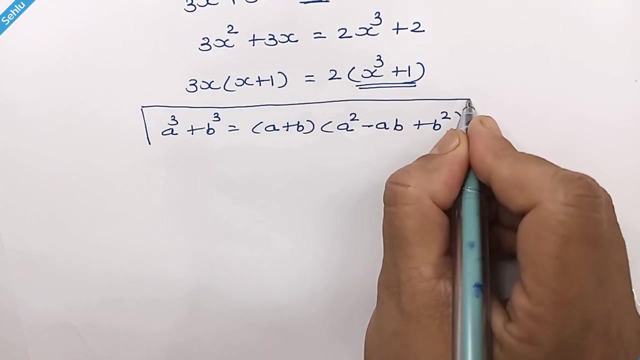 Factor out 3x from here, So it will be taking 2 common sides. For this part we can apply an identity of a cube plus b cube. then it can be a plus b times a square minus a, b plus b square. So here we can write. 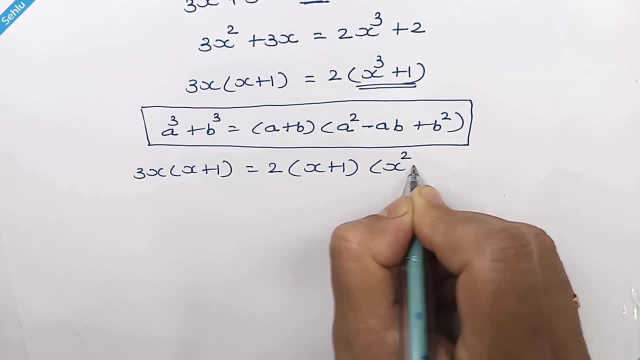 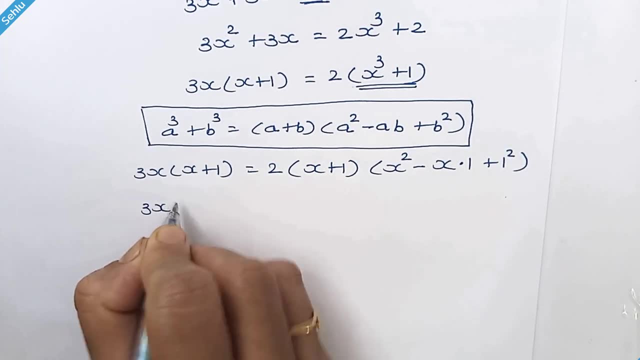 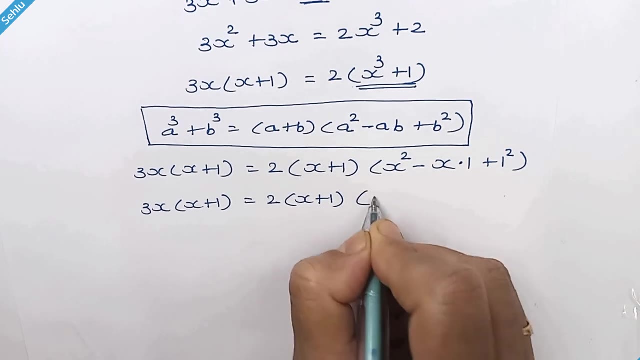 x plus 1 times x square minus x times 1 plus 1 square, Simplifying more. so it will be x square minus x plus 1.. Now we are gonna move this right hand side to left hand side. If we operate as it is, we might miss a solution. 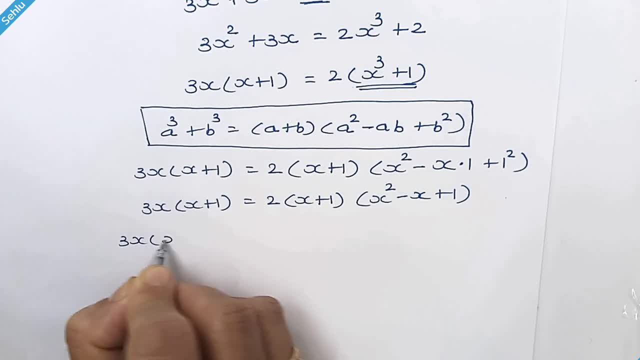 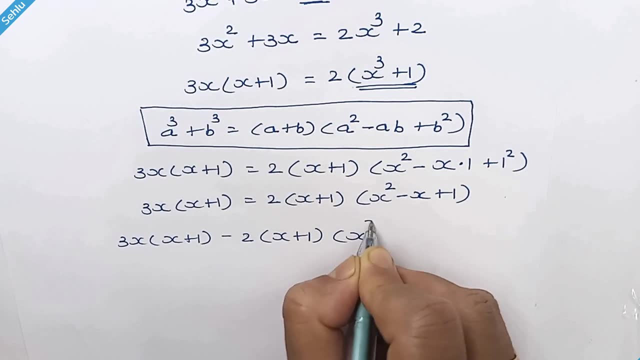 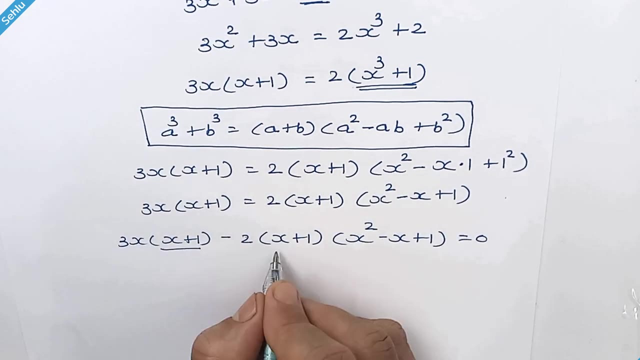 Simplifying more. so it will be x square minus x times 1 plus 1 square. We can factor out x plus 1.. So we have 3x minus 2 times x square minus x plus 1. So we have 3x minus 2 times x square minus x plus 1.. 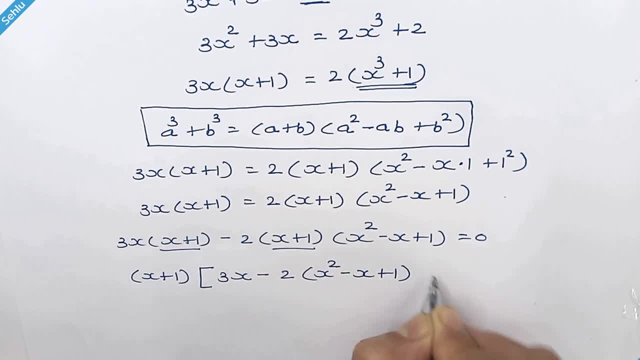 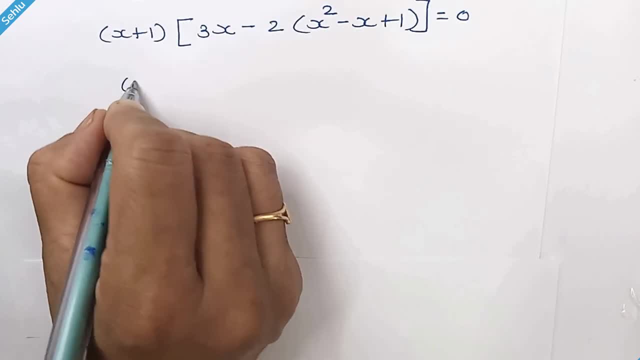 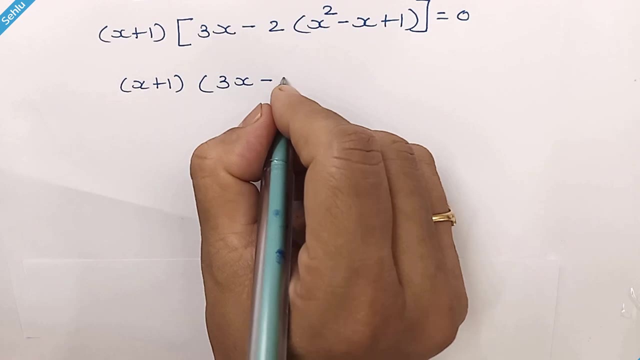 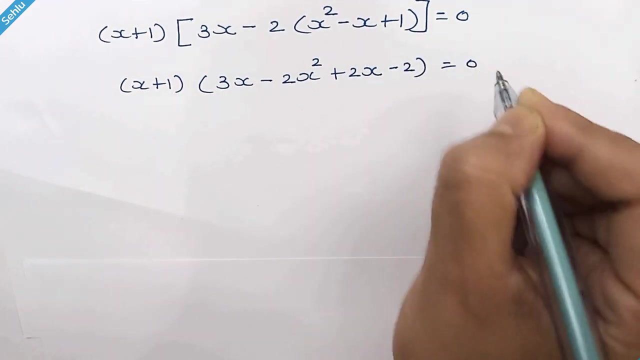 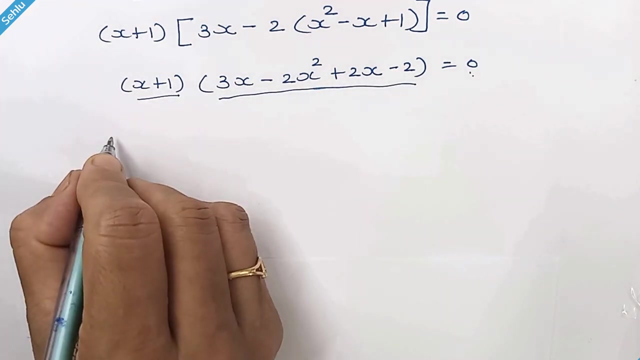 So we have 3x minus 2 times x square minus x times 1 plus 1 square x plus 1.. So in the next step we have x plus 1 times 3x minus plug in 2 into this bracket, so it will be 2x square plus 2x minus 2.. Now either this is 0 or this is 0. So we can. 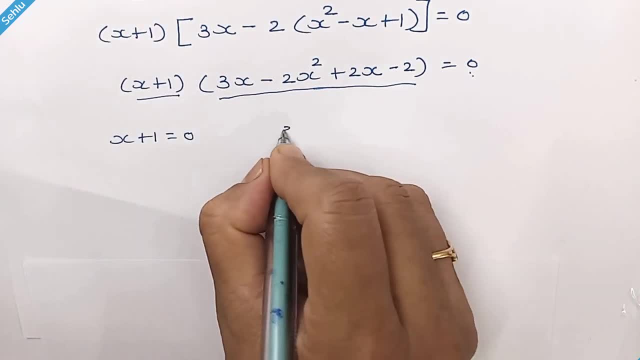 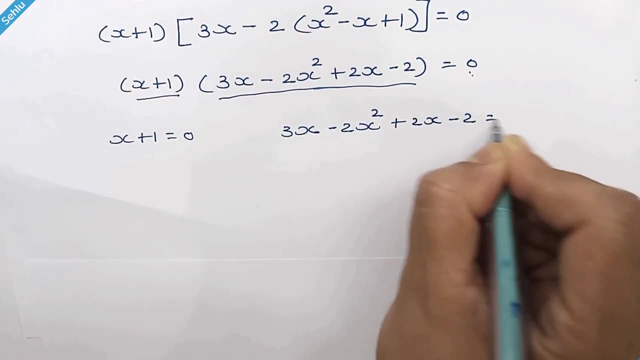 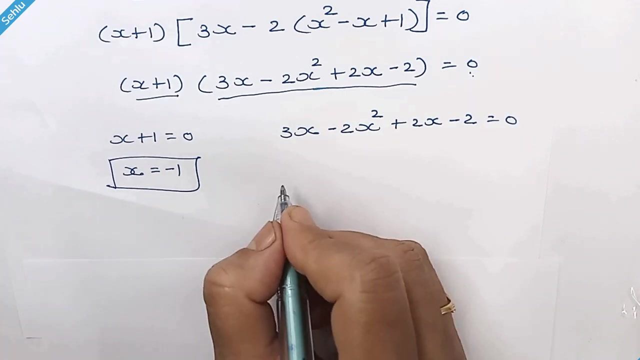 compare: x plus 1 is equal to 0 and 3x minus 2x. square plus 2x minus 2 is equal to 0. So here we have: x is equal to negative 1.. It's the first solution These two can summed up. 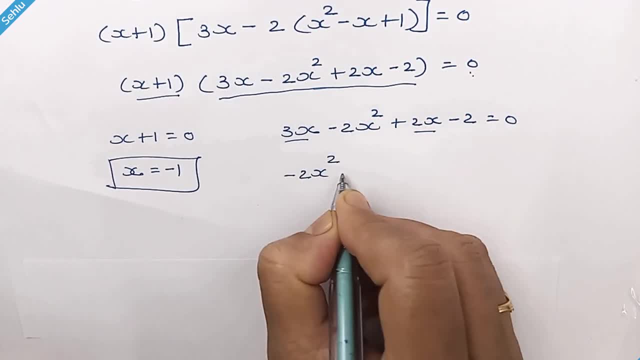 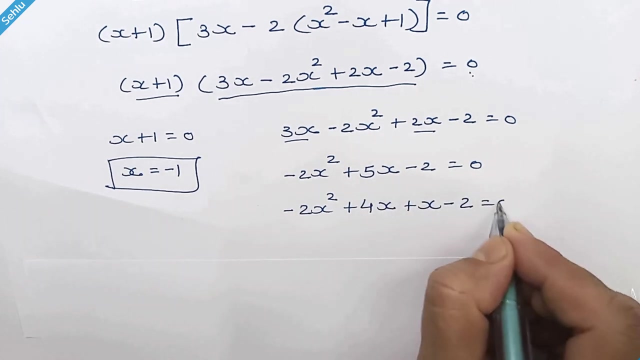 so we have negative 2x. square plus 5x minus 2 is equal to 0.. Now it's a quadratic equation we have and we can factorize it by placing 4x plus x instead of 5x. Factor out negative 2x, so it will be x minus 2 and here we can factor out 1.. 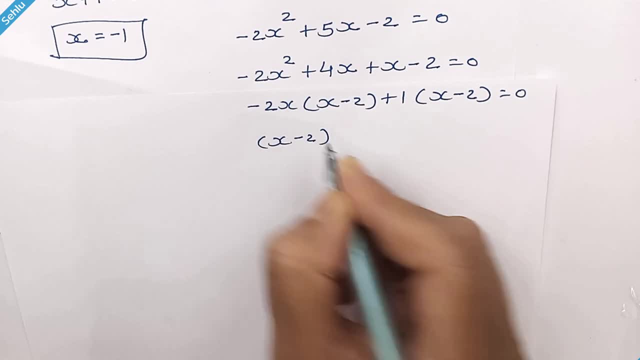 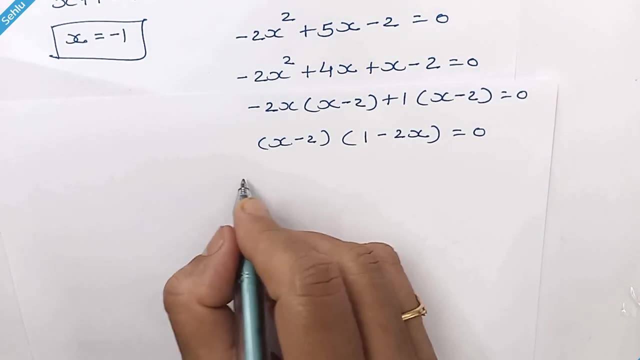 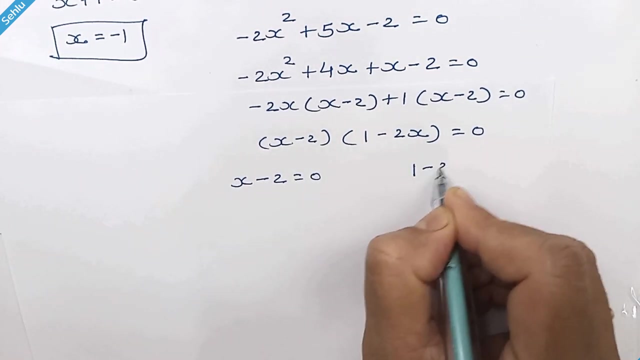 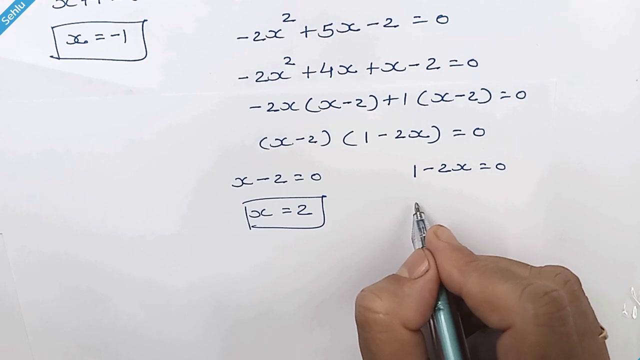 So we have x minus 2 times 1 minus 2x is equal to 0.. It can be: either x minus 2 is equal to 0 or 1 minus 2x is equal to 0. So here we have: x is equal to 2. And this 2 is. 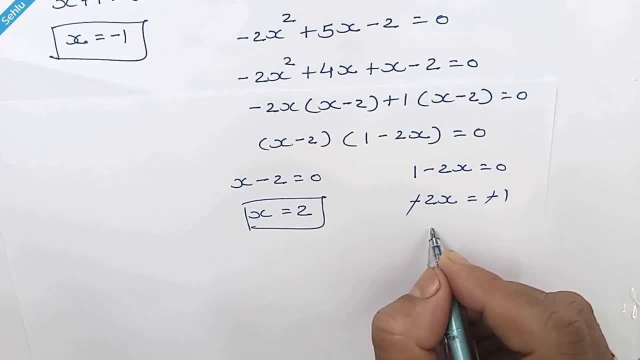 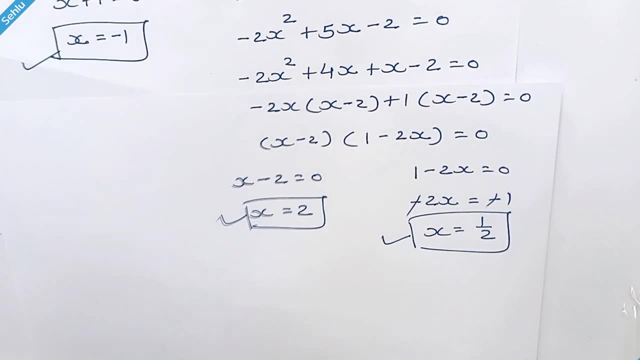 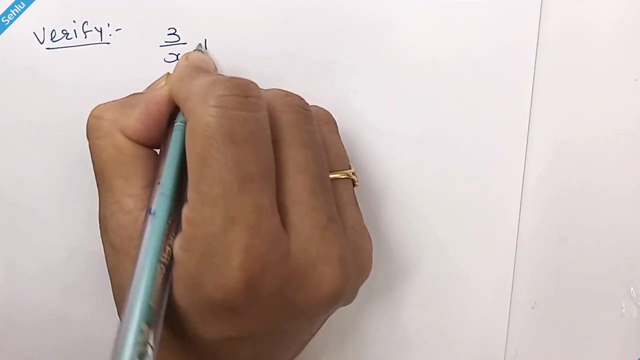 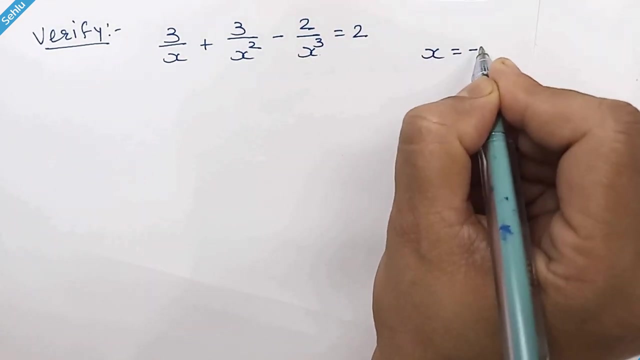 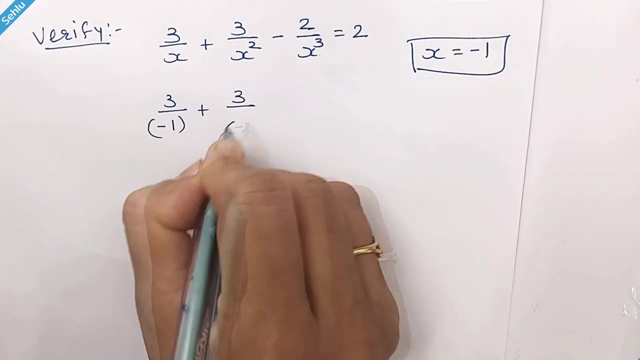 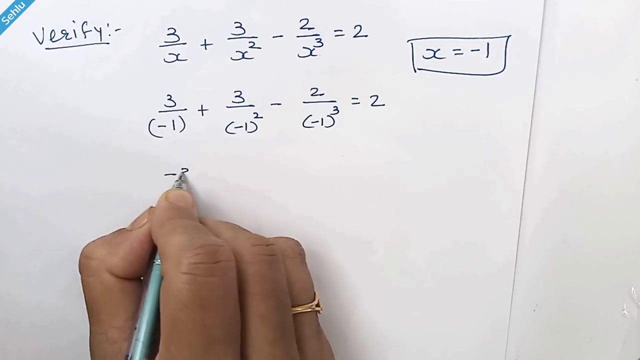 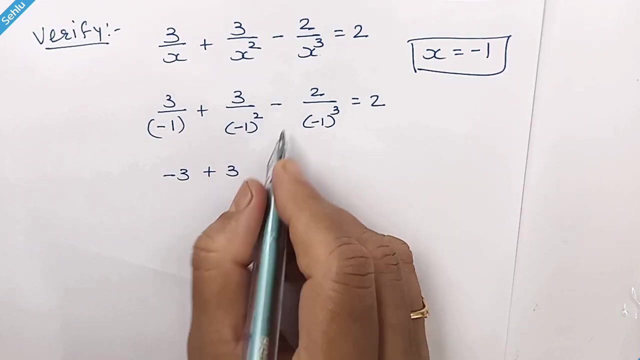 equal to 0. These two will cancel each other and we have: x is equal to 1 over 2.. So these are the answers. Let's quickly verify them. Question is: let's take x is equal to negative 1.. So here we have negative, 3. Negative, negative will be positive, So we have 3 and negative.